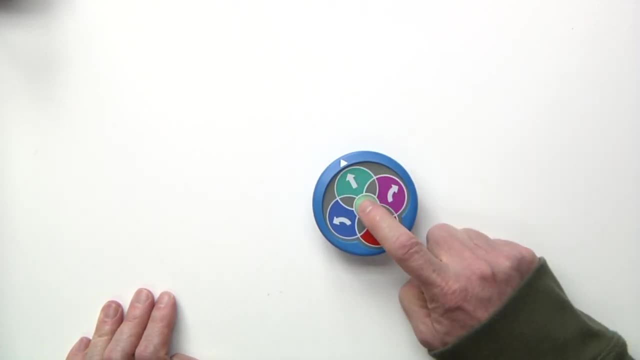 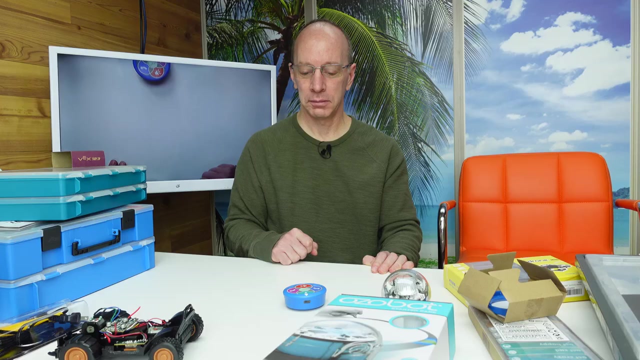 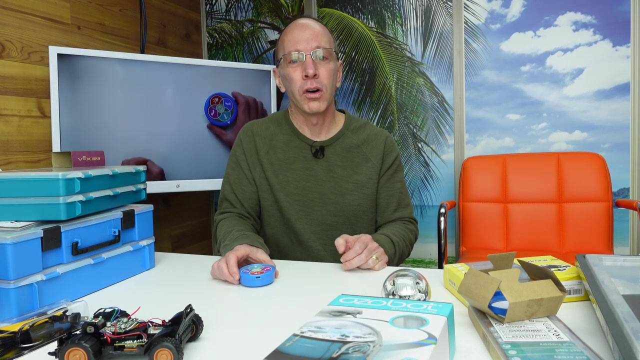 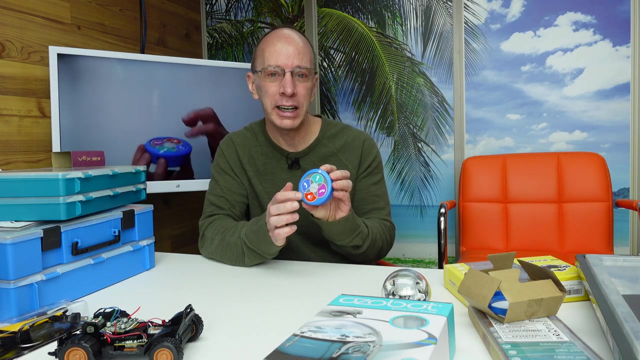 And then twice like that, And then you just hold down on the middle part And then there you go And all you have to do is shake it like this. So this is really neat because you can do the programming right here on the VEX-123.. But it also comes with a board with a lot of different. 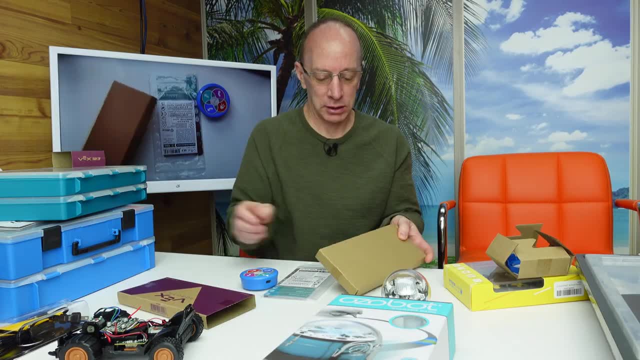 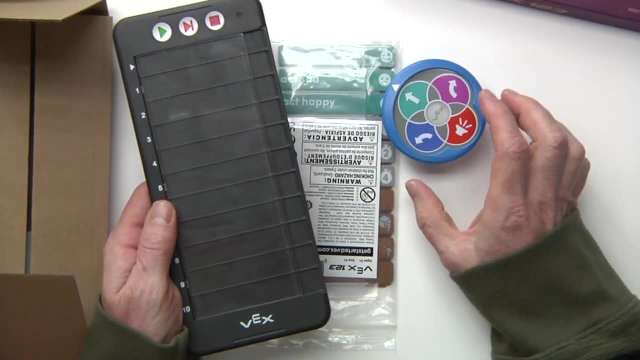 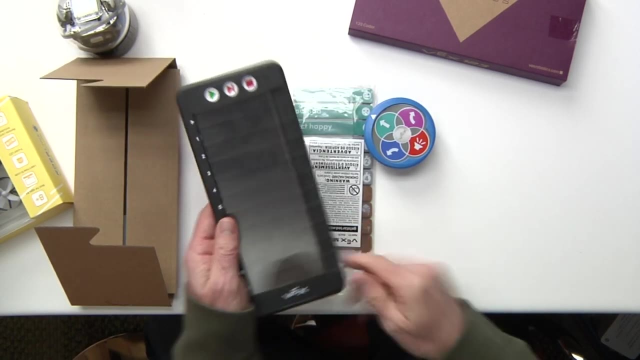 codes and commands there. So the board looks like this: It syncs up with this controller right here. Let me kind of zoom out here so you can see that It syncs up. It runs by two batteries right there And you would insert the codes And I'll show you what the codes look like. There's a ton of 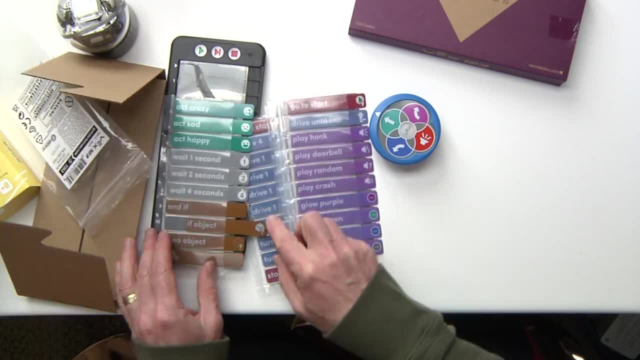 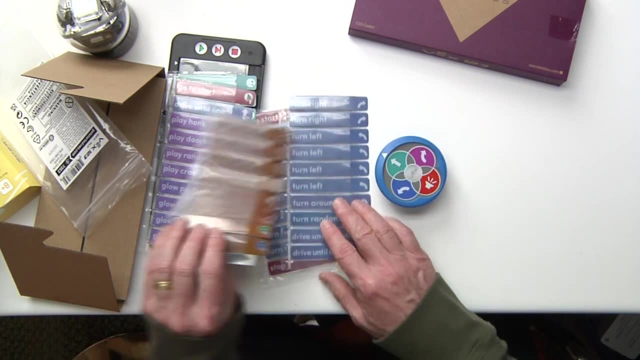 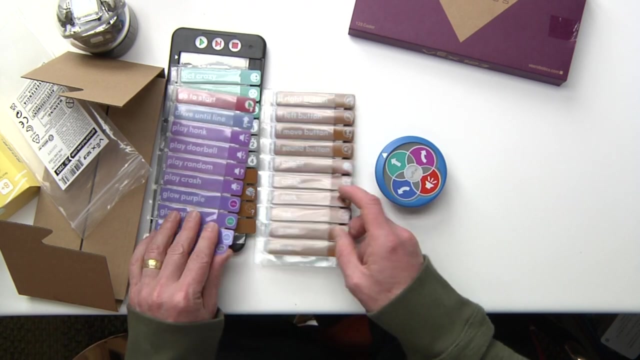 different codes right here So you can see that You can hit end if object glow, You can change the color of the lights on here, Turn left, Turn right, Random, Turn right, Drive. All these are really awesome And you just insert these codes right in here And you hit play And then that'll. 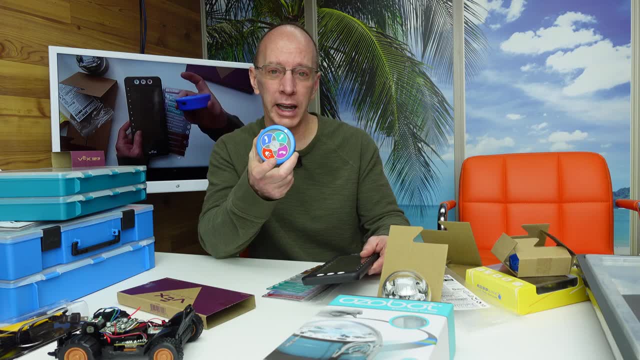 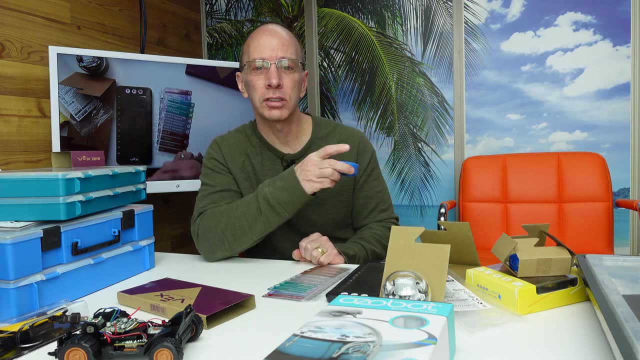 activate it. So there's Not only just one way to activate this. You can do it on this little hockey puck, You can use this board, But for your advanced users, you can also use the computer, your laptop, your Chromebook. 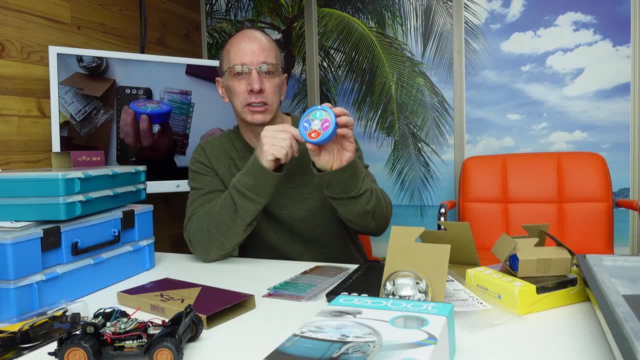 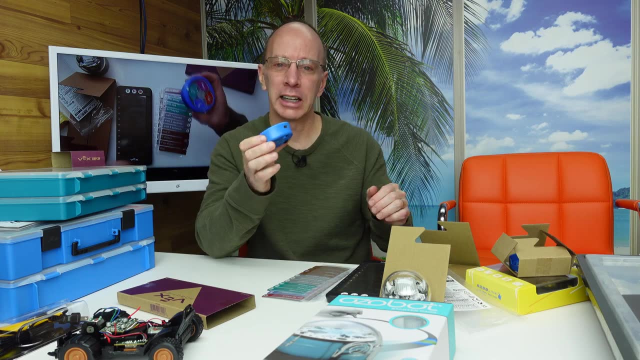 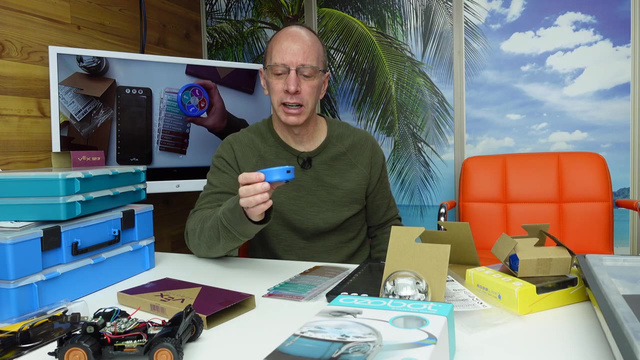 or even your phone to code with the VEX-123.. This is a great introduction to coding And I would probably recommend You know this could be great for like maybe a first grade or second grade With the VEX-123, it gets. It can get complex if you want to, Or it can get kind of. You know you can make it. 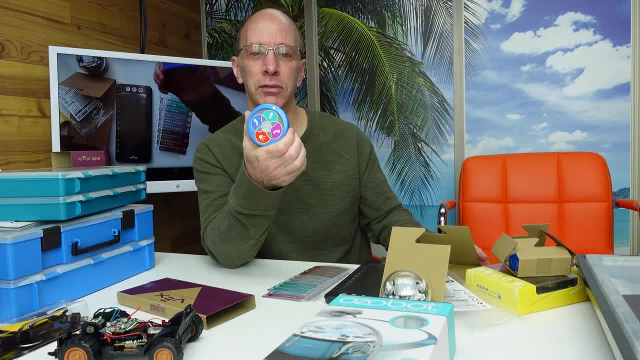 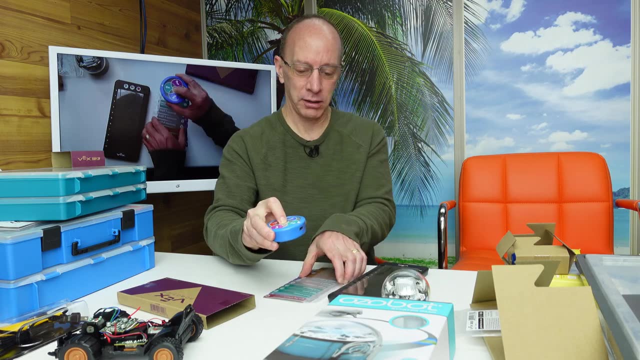 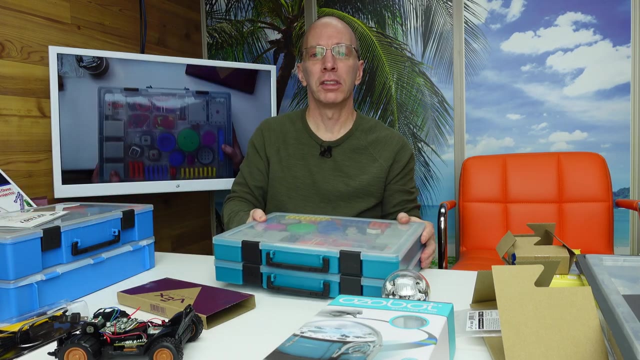 basic, But this is a great option for your robotic class is the VEX-123.. So I'm just going to go ahead and turn that off right now And put that to the side. VEX also has. It's called the VEX-GO Now. 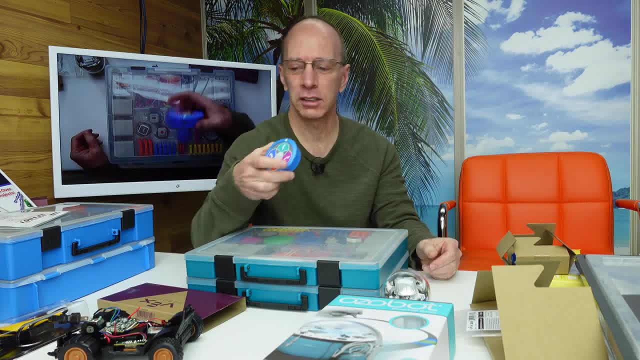 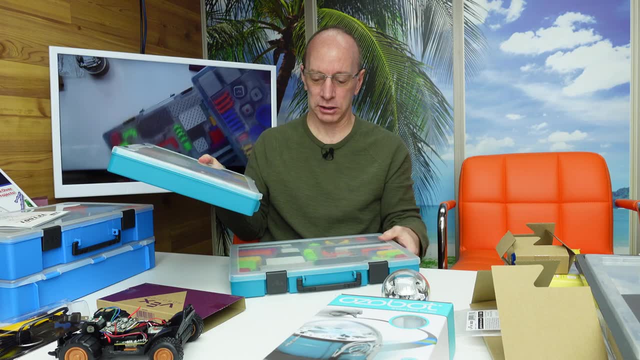 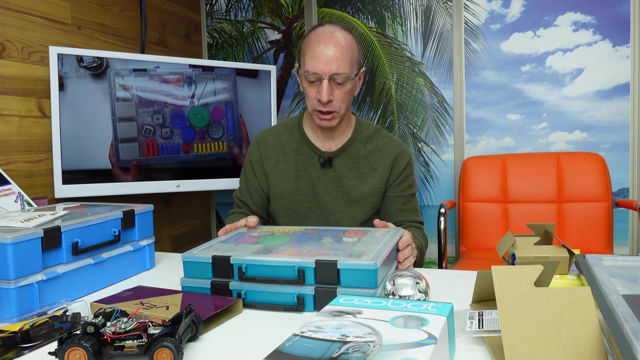 this one right here. this retails for about $120.. This, This is about $200.. This is the VEX-GO. It comes in two cases And it's designed to work with maybe two or three students. I like working with two students. That works best And it comes with a lot of cool. 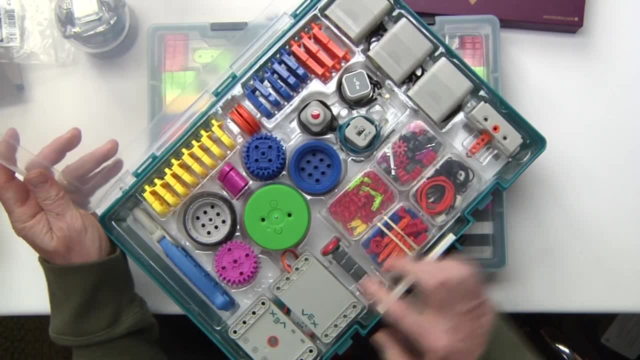 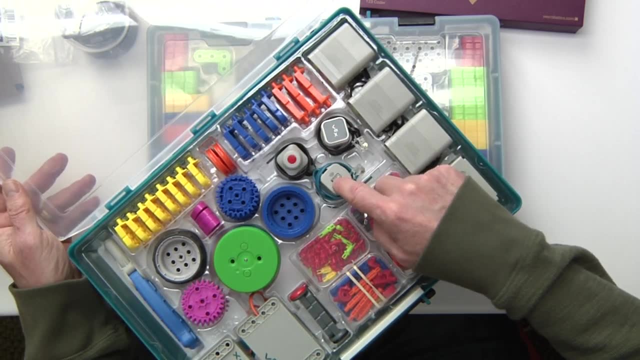 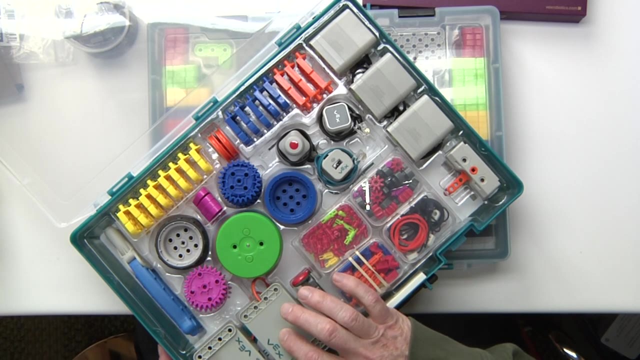 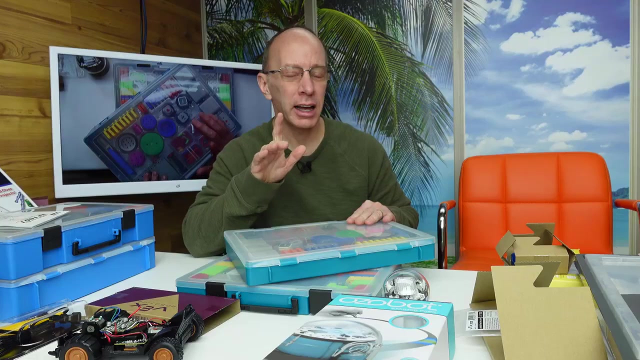 stuff you'll see in here. It has your motors right here, Your different sensors. It even has a magnet that you can turn on and off. It has light sensors like distance sensors. It has a rechargeable power pack and your brain right here. So it's, It's awesome And the way, The way. VEX. 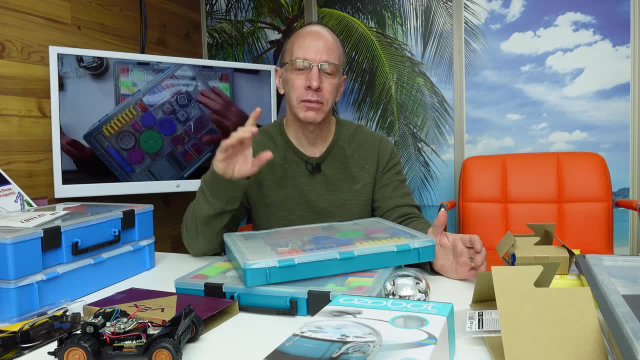 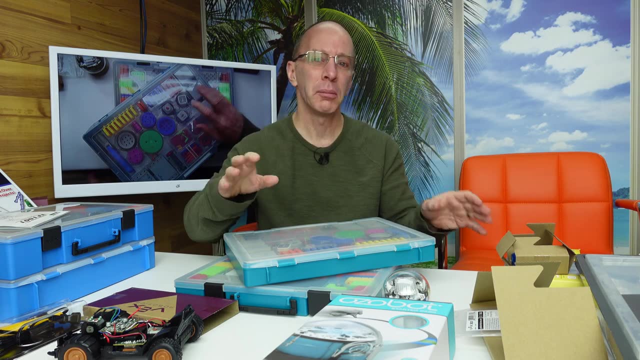 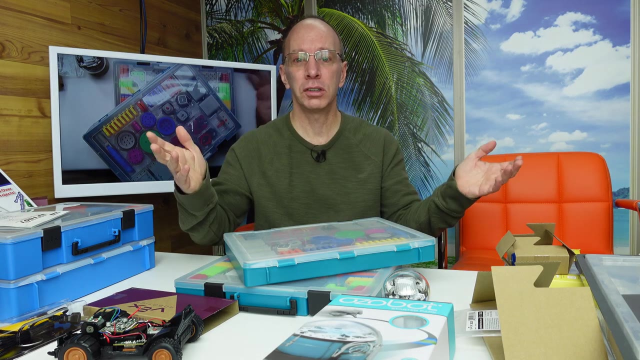 sets up their program is they have an awesome curriculum that works with the teachers, It works with standards, It's all set up. It works with engineering, literacy, mathematics, science, And you go in there and it's like a whole year long or two years curriculum on. 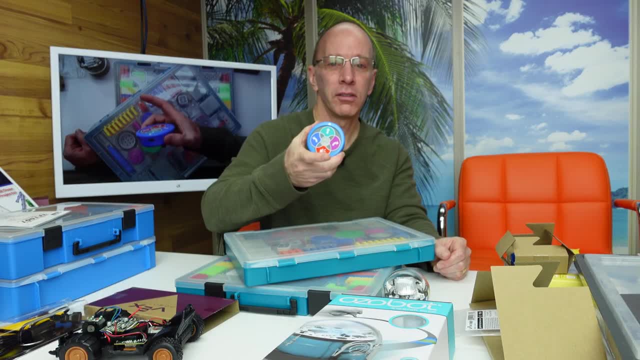 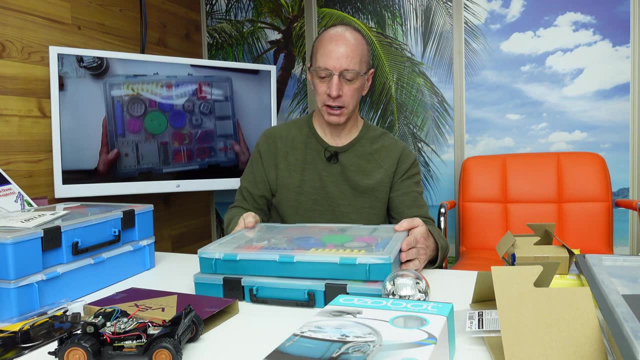 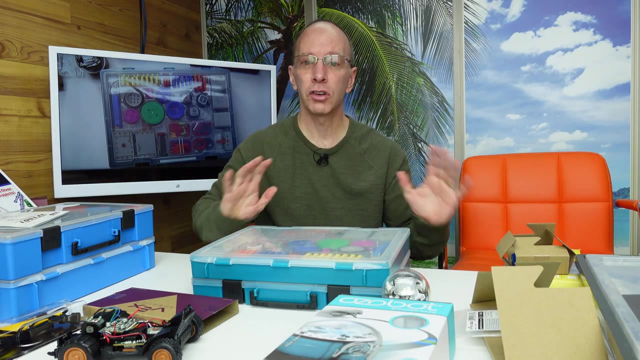 different things. they have a curriculum set up for the vex123, the vex go and even the vex iq and other vex products. this right here- i'm using this with third grade and third grade loves it. there's so many things to teach with. right now we're doing a lot of engineering and then we're going to get. 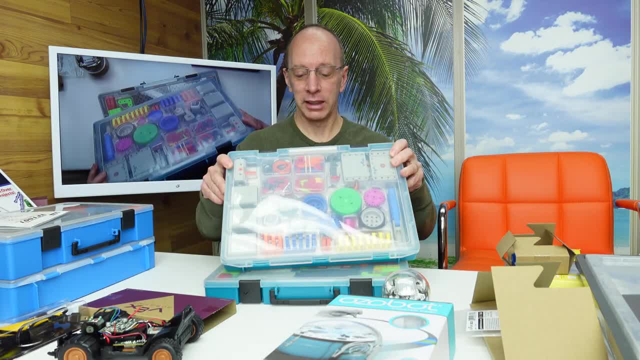 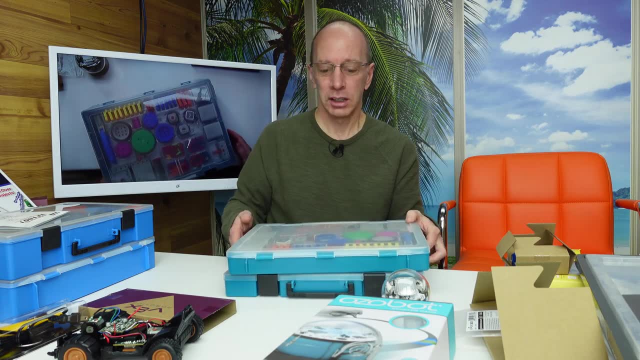 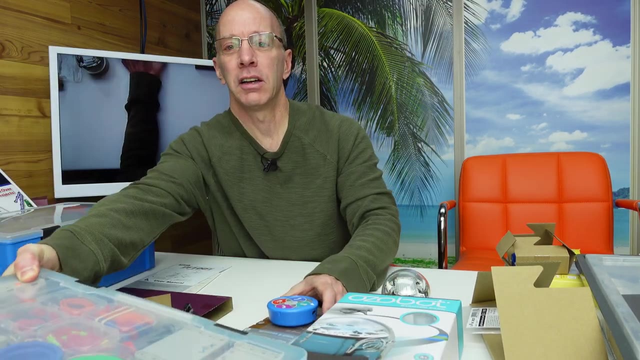 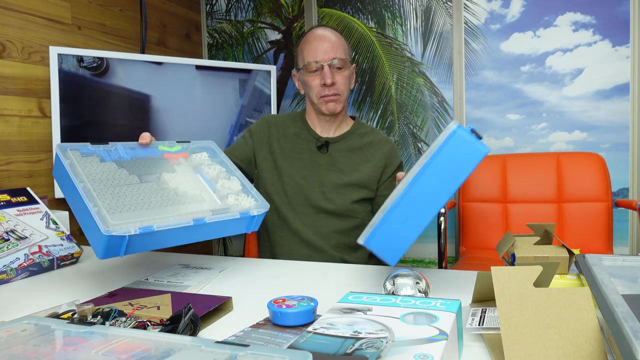 into the coding, so this is highly recommended. i love it, very easy for the teachers, a huge library of resources. so i'm going to put this off to the side here and i'm going to show you another product, and that is the vex iq. the vex iq comes in two cases like this. and the nice thing about 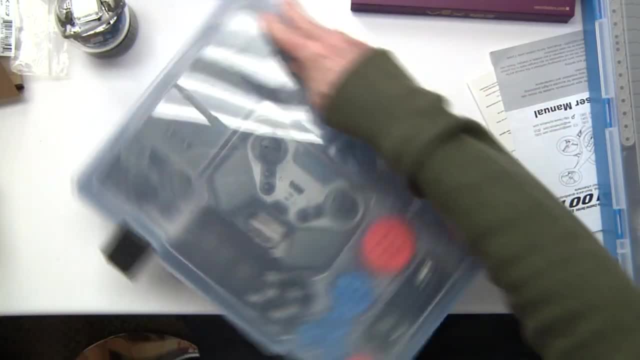 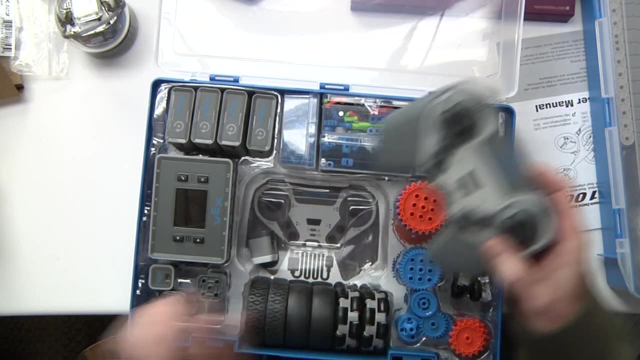 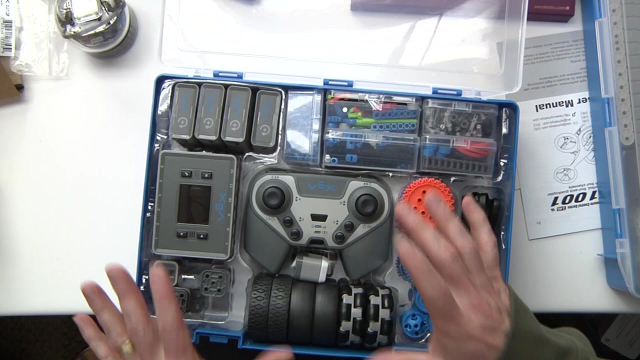 the vex iq is. it has a controller and it's a little, quite a bit more advanced with than the vex go. there's so many vex products. i'm kind of getting them mixed up a little bit, but this is probably geared. i would probably start this maybe in fourth grade, but there are schools that start it earlier and they just, you know. 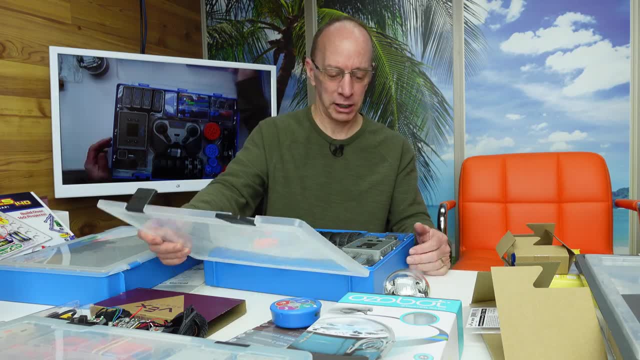 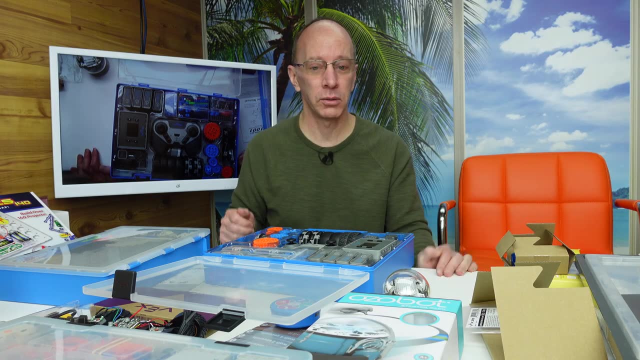 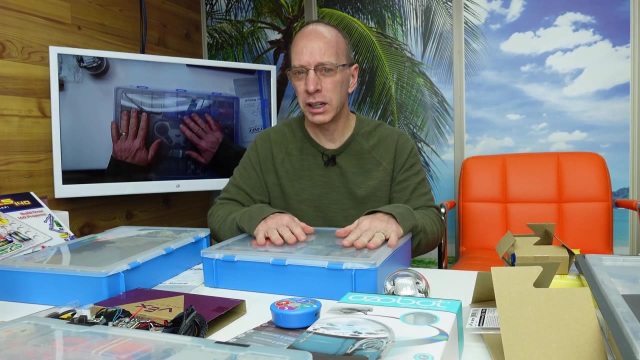 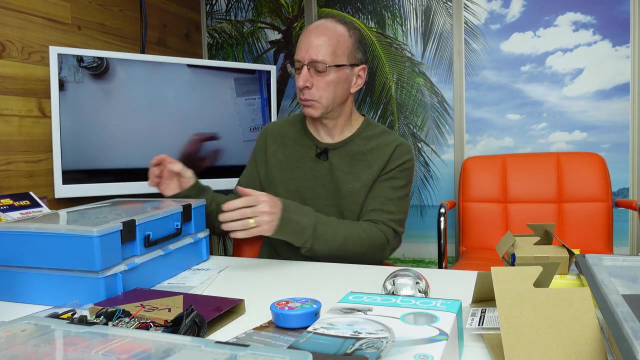 adapt it to their curriculum and the student's learning ability. this is really neat. check out on the vex website. you'll see like it's just amazing what they're doing with the vex iq and there's competitions and everything is set up. so this retails for 450, i believe, and once again with the vex products like this. 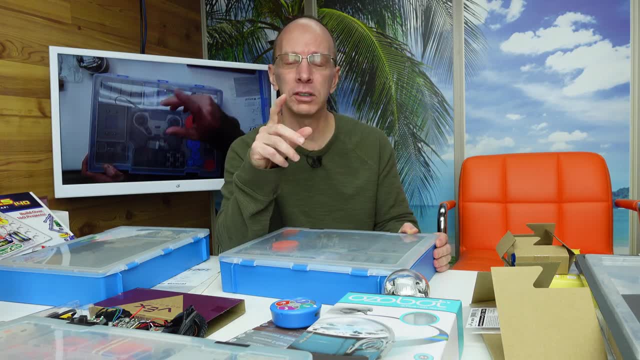 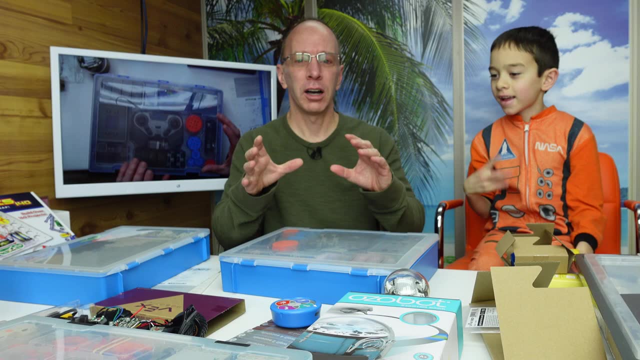 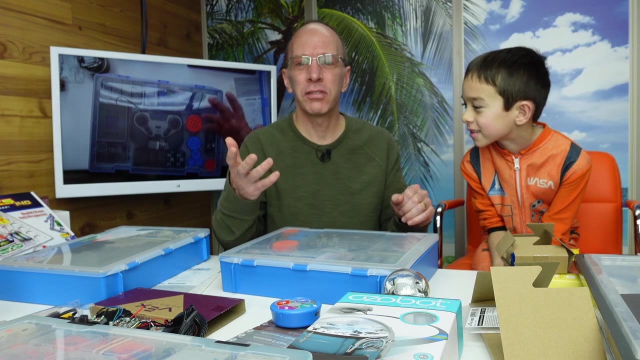 in the vex go or and even the vex one, two, three. it's designed to work with maybe two or three students, because you will have a student that they have different responsibilities. the cool thing about vex is it's designed it's like about 45 or 50 minutes and halfway through. 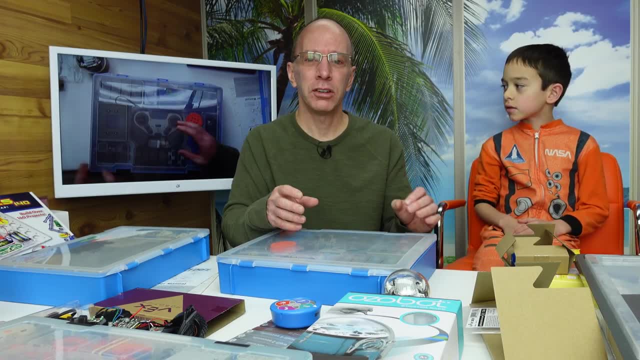 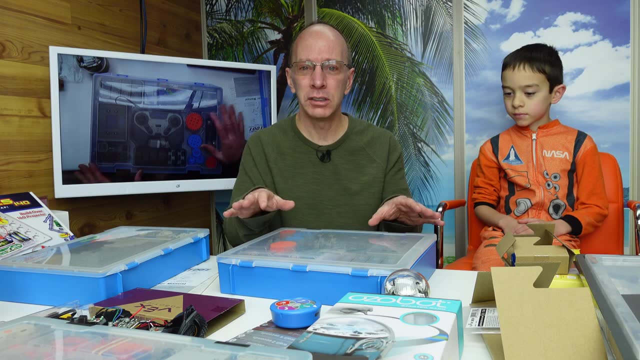 you take a break, you have a meeting and you discuss problems and you do a lot of problem solving, thinking outside the box. how can we solve this? how can we make this better? what can we do different? and then after that, then those two students are going to switch. 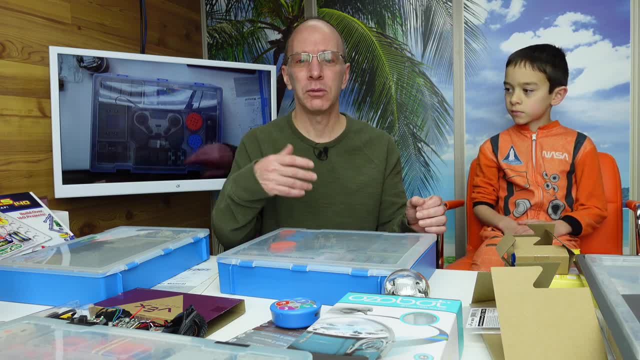 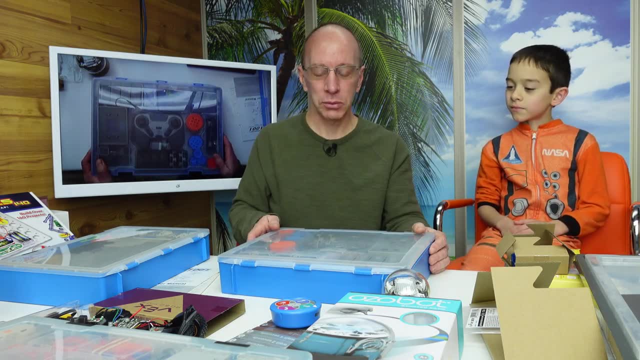 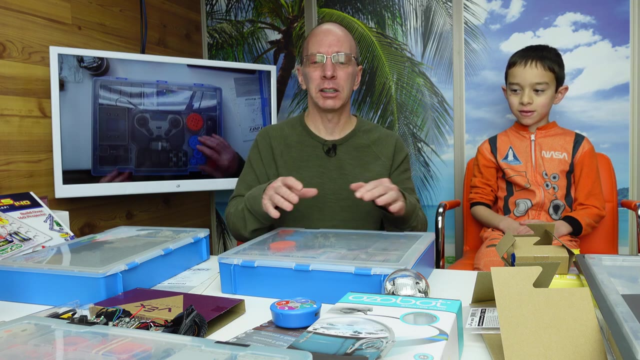 their responsibility, and now one is going to be the builder and one will be the designer or you know whatever. uh, you switch them controller. so, um, it's, i love how they set it up and then, at the very end, you want to allow a little bit of time to, you know, put things back into the case. 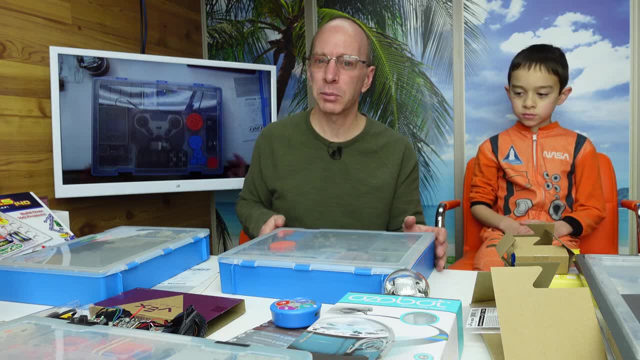 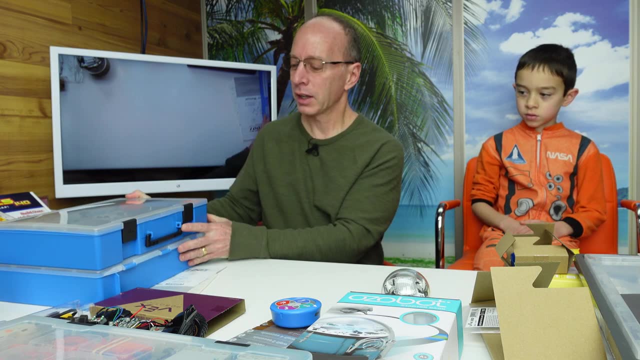 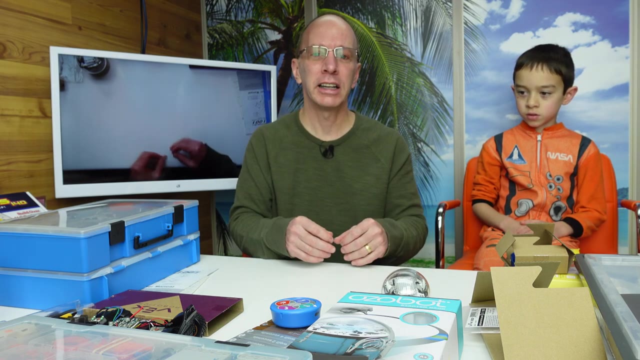 and break it down if you choose to. sometimes when you do some complex problems with complex models or building with the vex iq, then you can just keep that for another day. but these are set up that you know when you're using your vex kit you you have time to put it back together, and so you're. 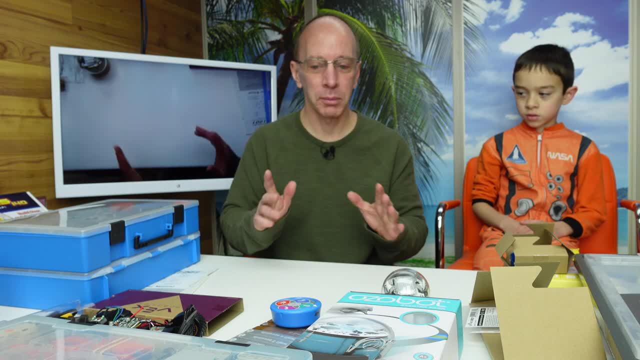 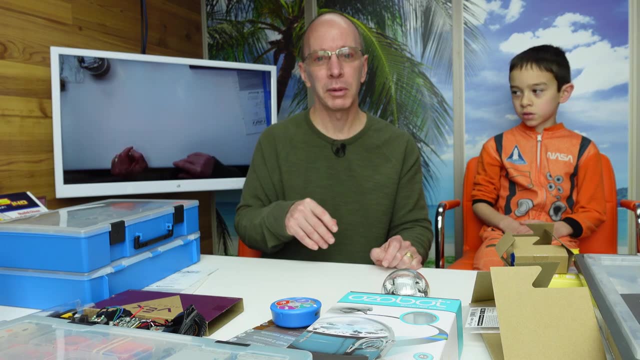 ready for the next class, and so, um, awesome, awesome, awesome, um, like i said, vex, um, there's another one for high school. i don't have that right now, but, uh, that's, that's one of my goals, but uh, so we have the vex. uh, one, two, three. 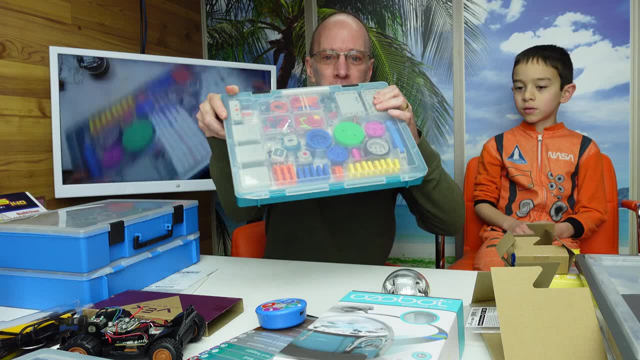 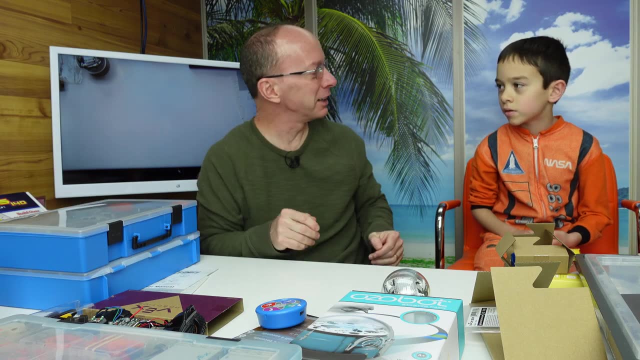 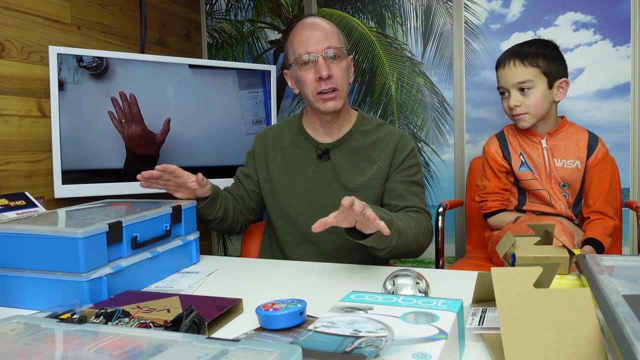 the vex go right here and the vex iq, so we're super excited. good morning there, lucas, how you doing? my lucas has a kind of a cold right now, so all right, the this is great. i love working with the vex. they have an awesome curriculum, but there's some other robotic. 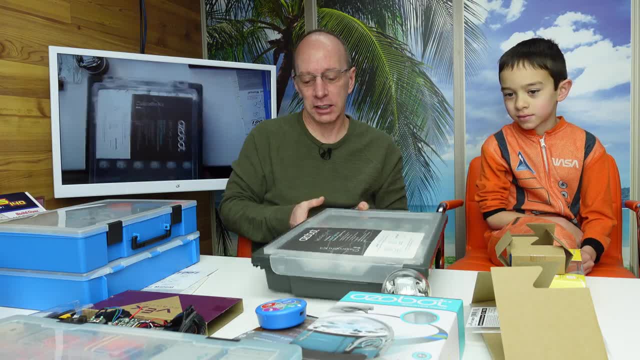 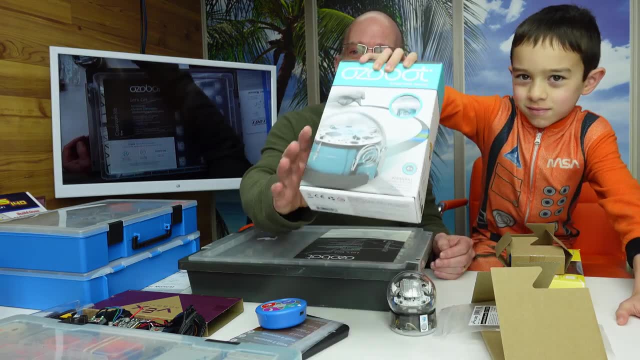 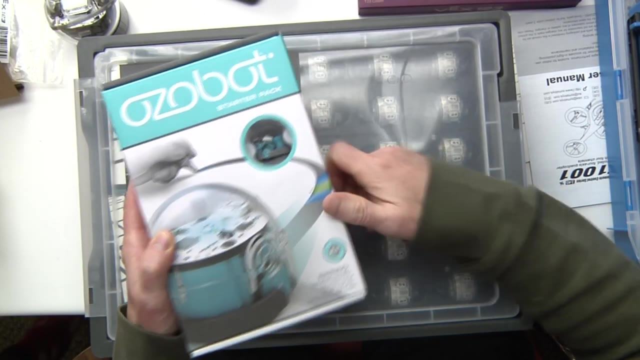 uh kits that i want to introduce you to. this is the ozobot and if you're ever looking, if you know, maybe you can go on facebook and see if anybody has some used ozobots. this is the ozobot bit, which is nice, but if you're going to be doing the classroom, i would probably get the ozobot evil. 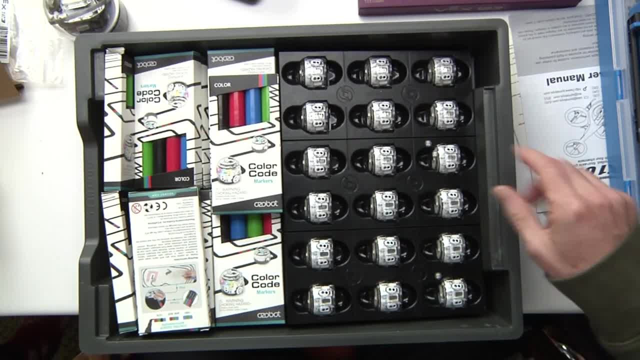 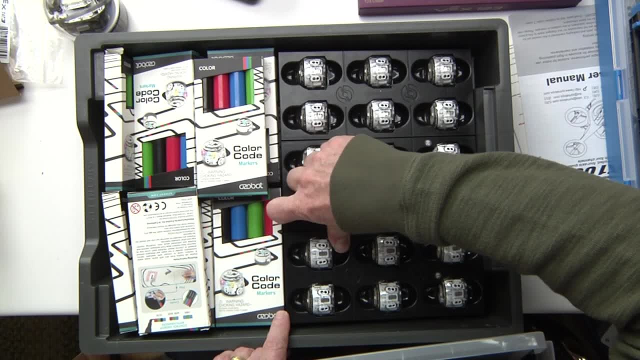 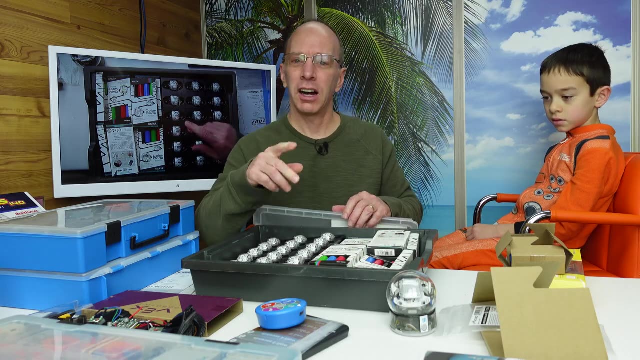 each. so this whole kit is probably about two thousand dollars. um, they come with markers. um, they come. uh, this, the classroom kit, is awesome because, yeah, you can, you can put them right inside here and snap them and charge them up. these are awesome. they are designed from kindergarten to 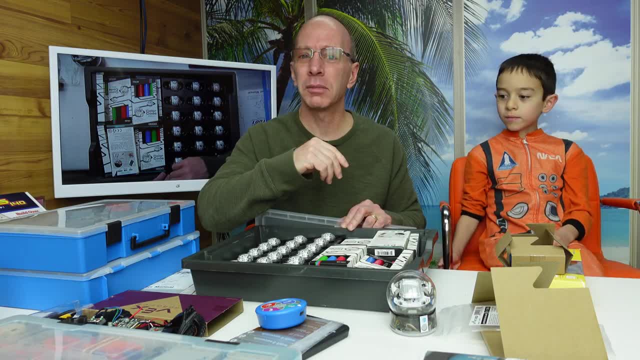 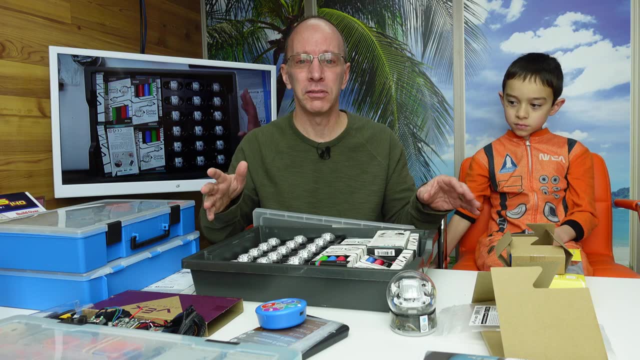 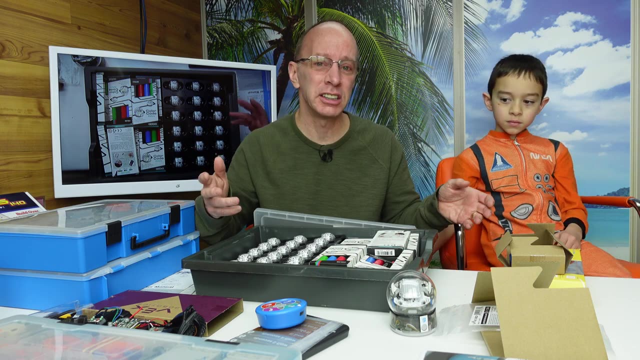 12th grade. they have an awesome curriculum also on their website. check it out. they have just like vex um. uh, the lessons are sometimes in vid. uh have video lessons um working with everything I'm talking like mathematics, science, history, social studies, uh literacy, uh verbs, uh compound words. 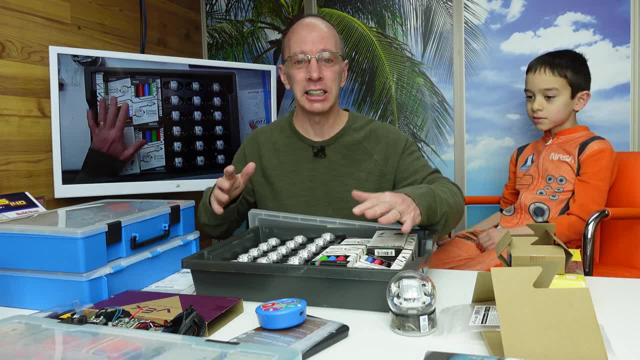 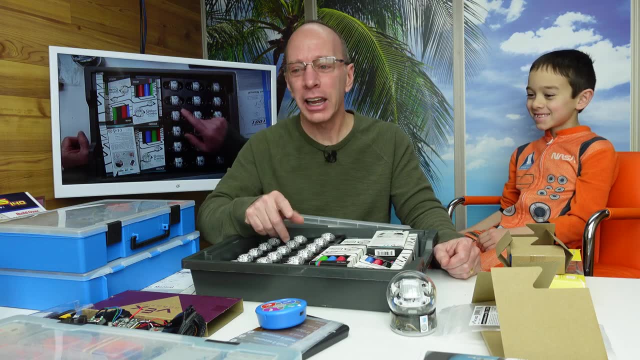 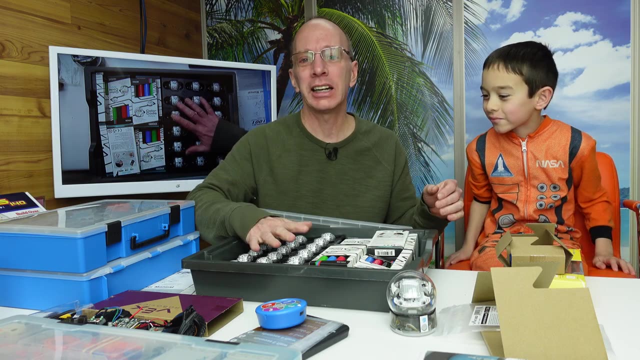 reading it's, it's amazing and it's con and it's just growing and growing. um, is that lunchtime? yes and uh. what I like about is, if you're teaching vex or whatever a robotic class you're teaching, mix it up, you know, bring in ozobots, bring in some of these other uh robotics that I'm going to. 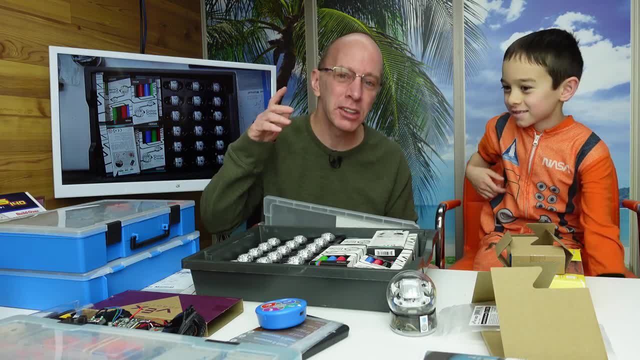 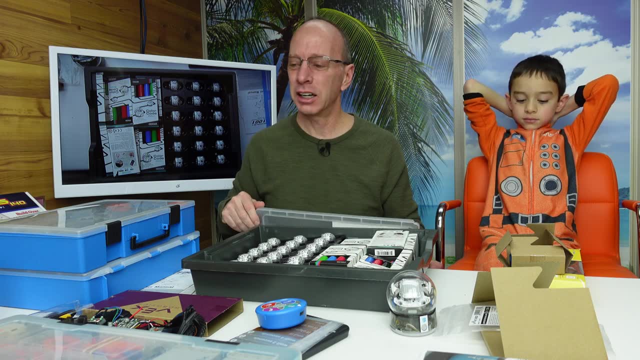 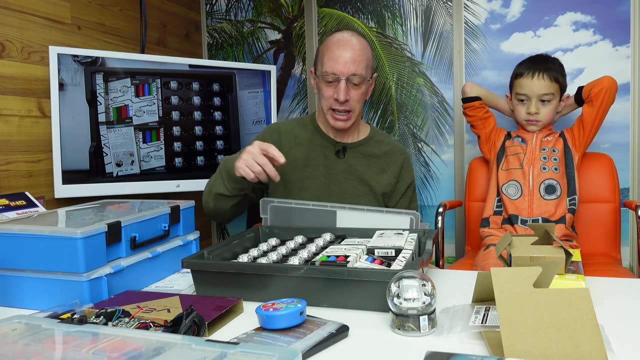 introduce? yes, because you're dealing with coding and it brings that level of excitement. uh, for me, if you're going to teach robotics, you want that excitement because, uh, you, you and and you want to change things up, so you want all those students to be involved and excited about this anyway, um. 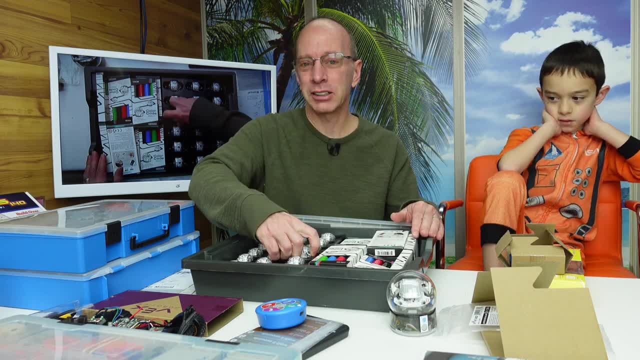 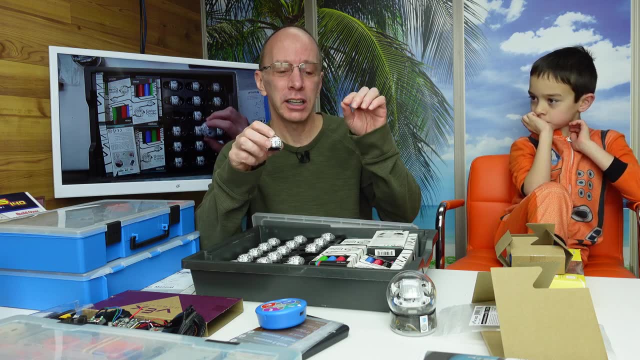 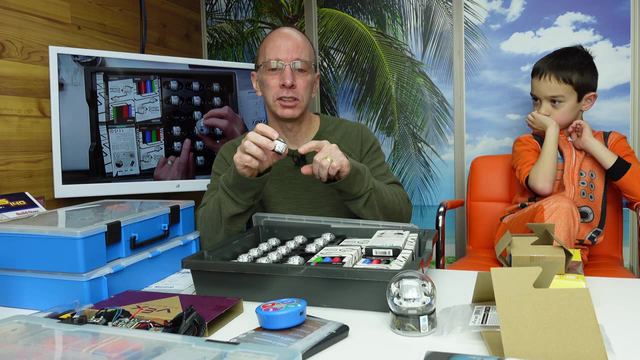 with the vex robotics, it's, it's um, not vex robotics with the ozobots- um, it's cool because they can follow a line. but it's not just about following line. you can use the markers to design your own code on here, and then you can also use the computer to code and 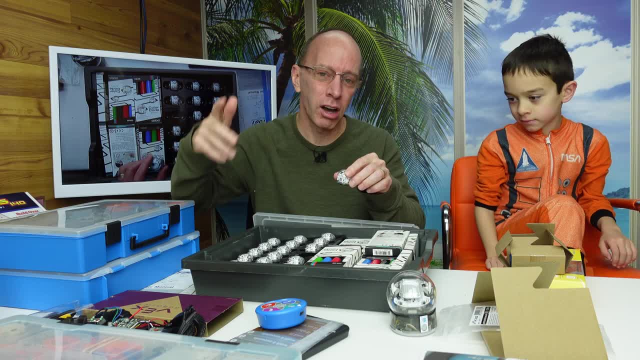 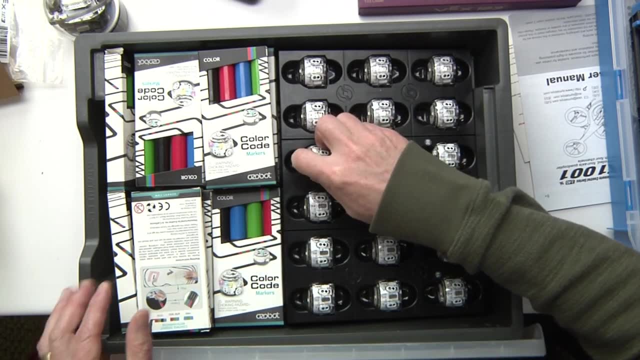 then- and it's cool because ozobots has different levels of coding along with vex and these other programs, so it has your basic coding and then it works into more advanced coding for your other students, like even in high school. I'm not going to go into a lot of detail on the ozobots, right. 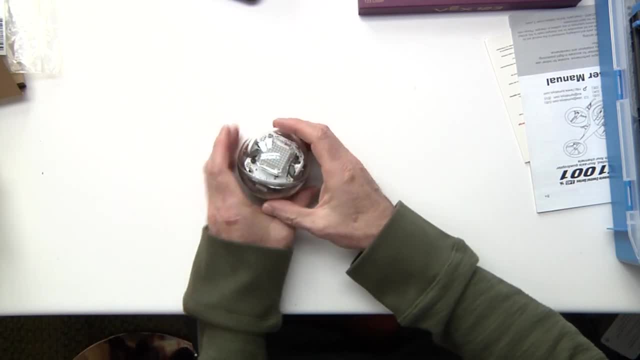 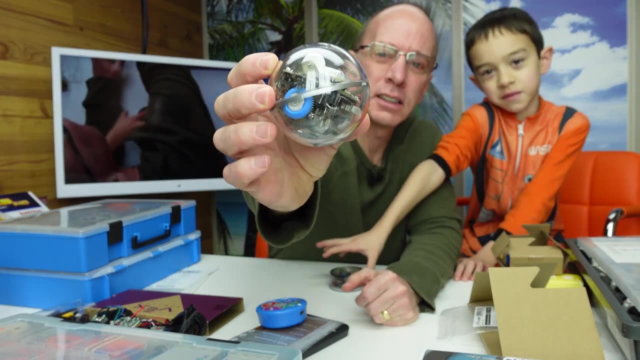 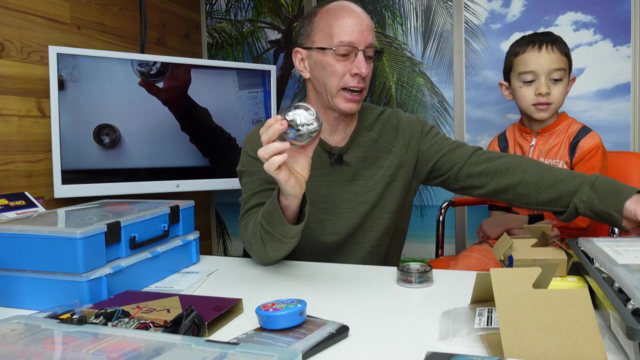 now, and I'll also make a video on this. the next one is called the boat. it's the uh both sphere and this is really cool and this comes with this. yeah, it comes with that. that's his child and this is waterproof and this is extremely fast, so I'm going to do a um, can you go right through it? can it can? 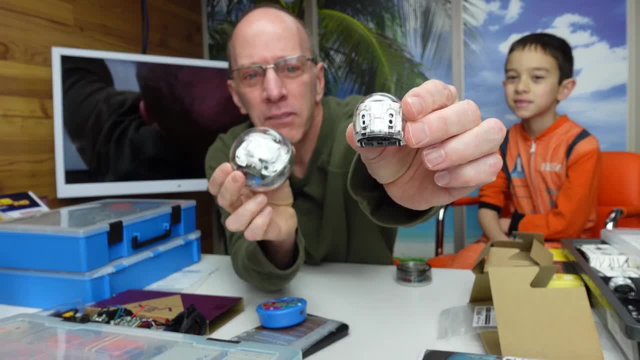 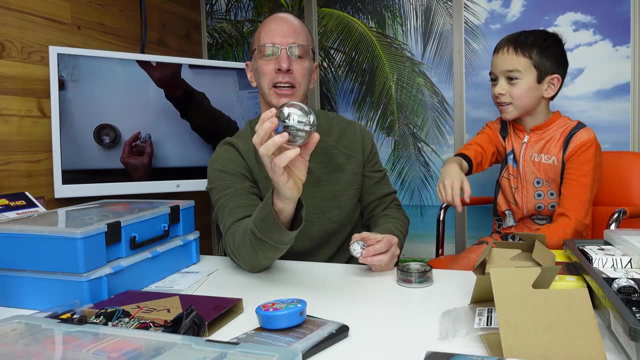 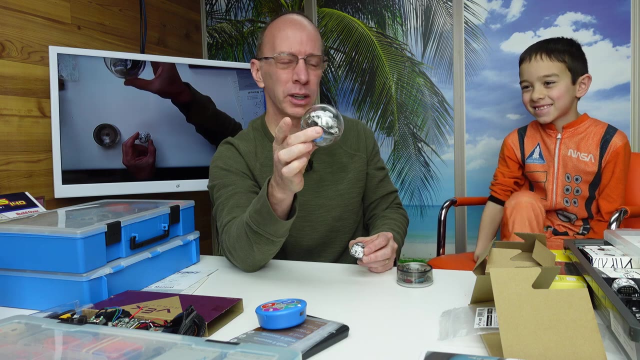 go right through the water. so, like I said, this is an ozobot and this is the sphere. bolt right here again. just chase a boat. I don't know if it can chase a boat or not. again, with this company, they have some other robotics um on there, really cool um, I think it's like a car or something like that. 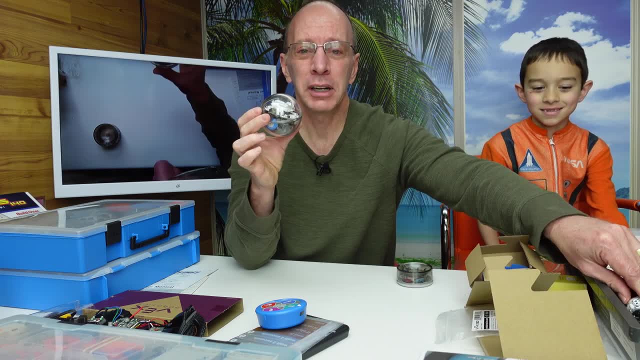 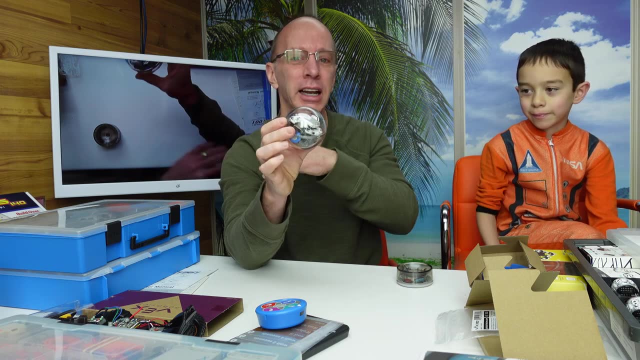 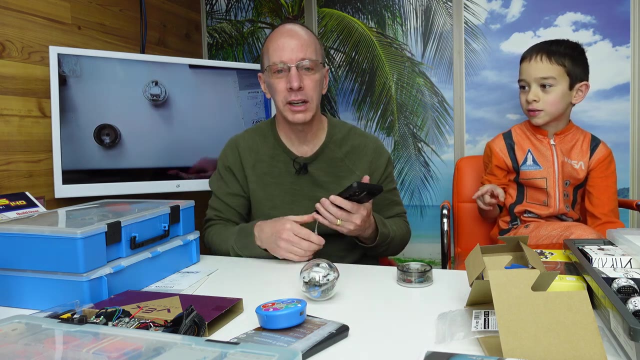 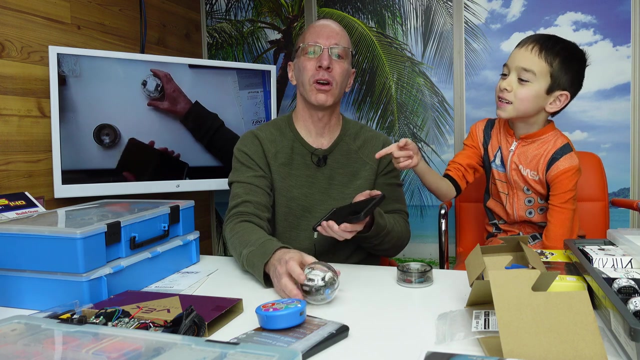 I'm hoping to do a review on that again- a company that has taken time and has an awesome curriculum set up for the teachers, going from mathematics, science, literacy, everything. and the way this works is you um code it? you can use your phone. uh, you can code it. yes, you can kick it. you can program it. code it, uh, you can use your phone. 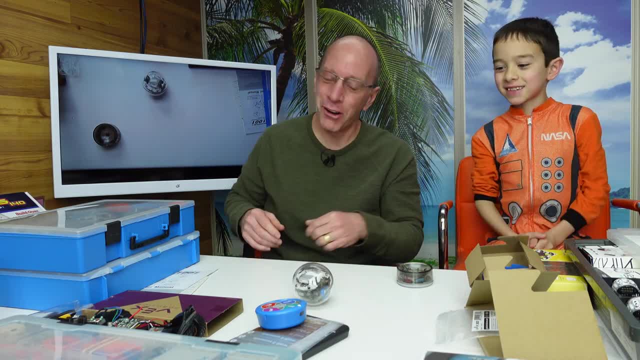 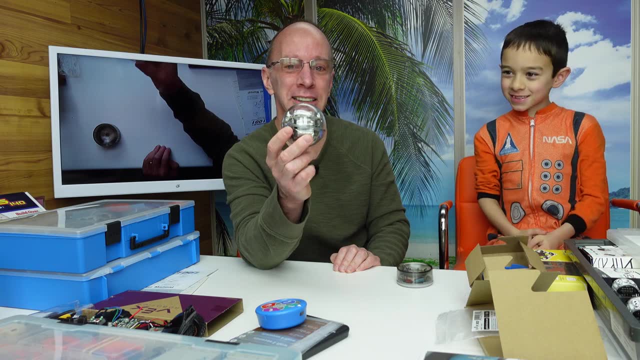 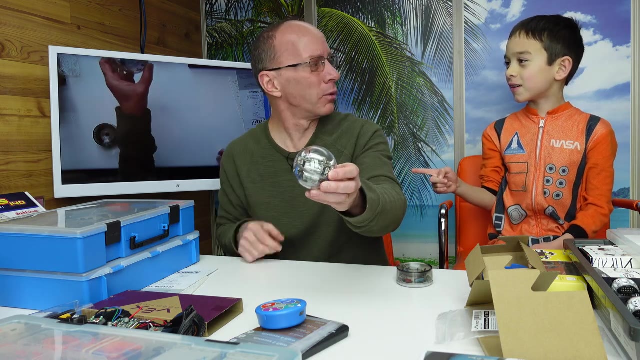 or the computer, you can hot, you can tuck it. no, you can't hit it. no, no, on the phone, yes and um. the other day, uh, Lucas was using this um in the school and this thing went so fast down the hallway. so, um, oh, was I doing it? yeah, oh, okay, that okay. and uh, make sure you check out my channel and my. 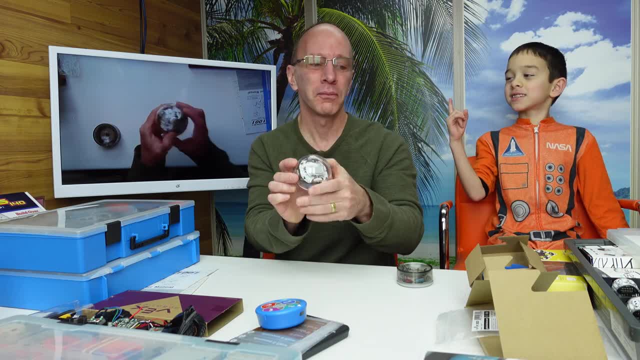 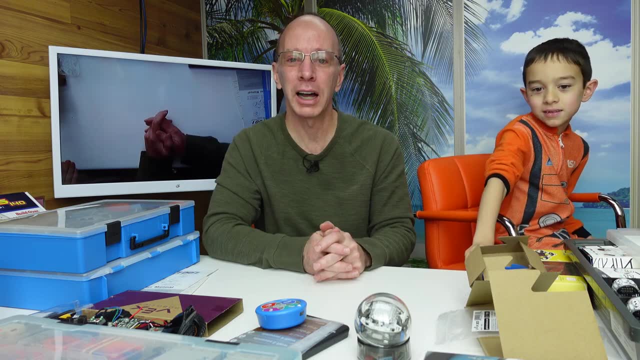 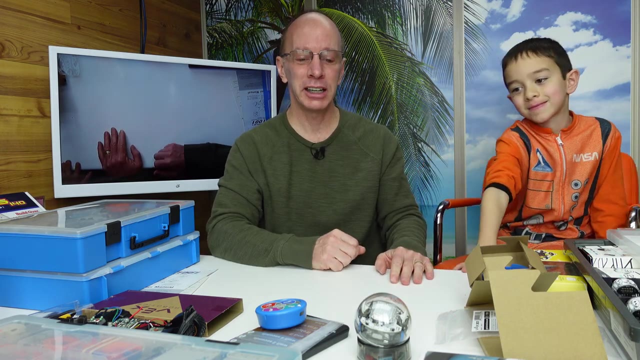 videos. I'll have an awesome review on this, and it wasn't yesterday, but this is an awesome, uh, another awesome thing to introduce to your robotics class: um, because you're, you're, you're, you're shaking up your class, you're adding the excitement, bringing in new things. another new thing: where is it I got? 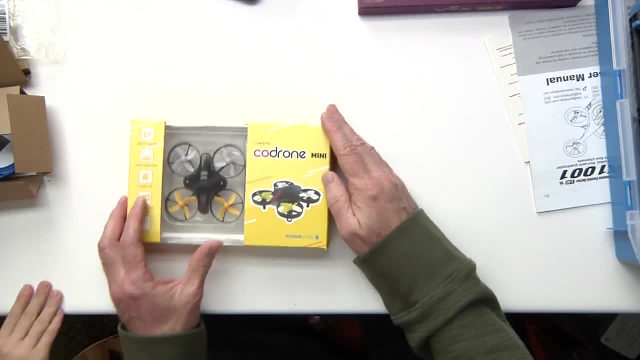 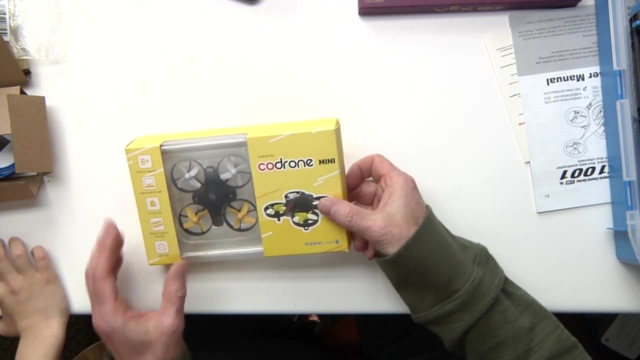 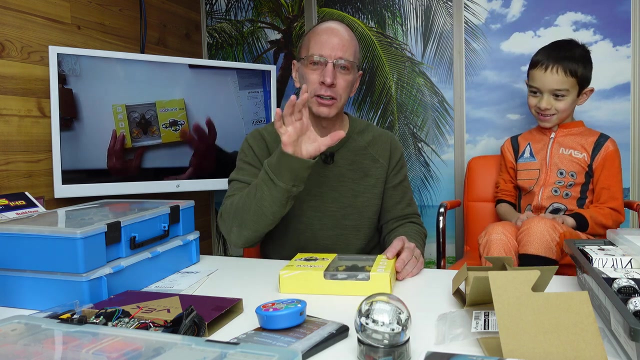 so much stuff right here. this right here. this is code drone. check out my video. I have a video on this. this is not like your regular drone that you're going to have at Walmart or a cheap thing. oh, going that way. well good, are we putting on a new show? yeah, we got a lot of drone videos, but this is not that. this is made so that. 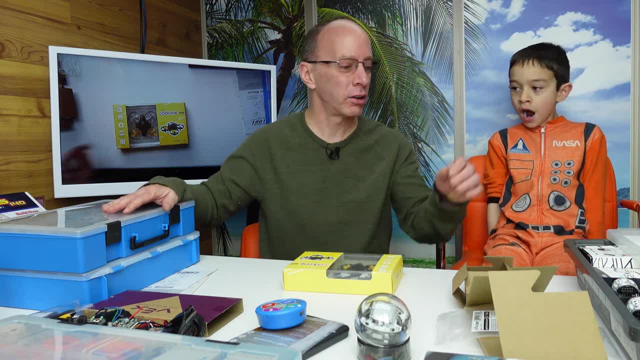 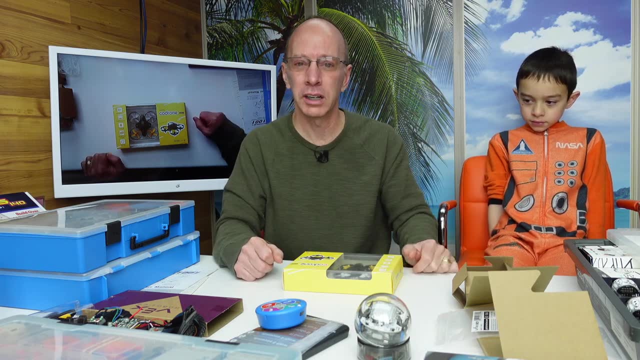 you can code with it. so once again, when you're coding with vex, you're coding with azo about, you're coding with the boat sphere, why not bring in a drone? a lot of schools are going to toward drone programming on coding and this is a great starting point because 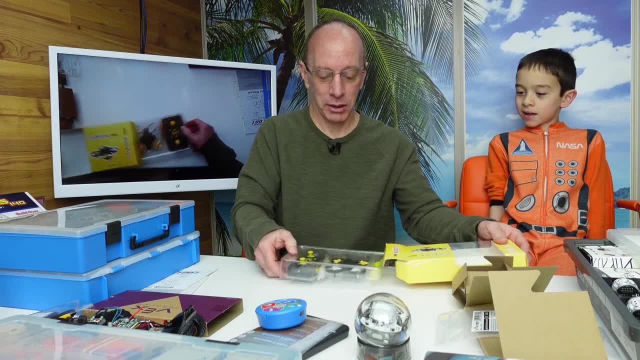 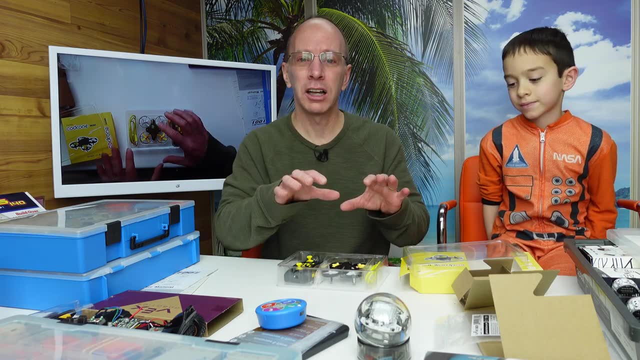 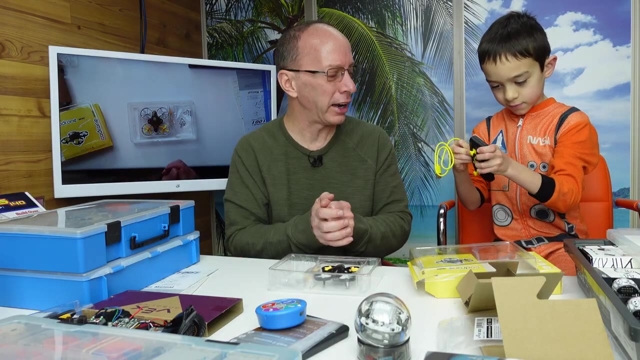 this is awesome. it really is. um, check out the video. I just I don't have a lot of time to go into it right now, but what you do is you go into the- uh, the program. I think it's like blocky code or something like that. again, blocky code starts from basic and you can also have more advanced. 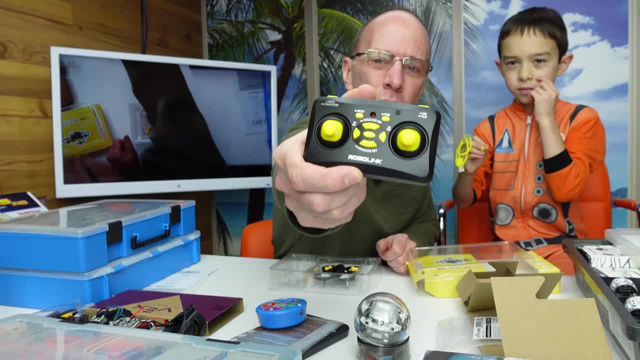 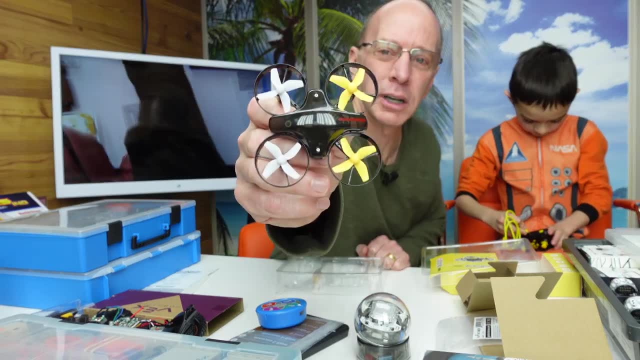 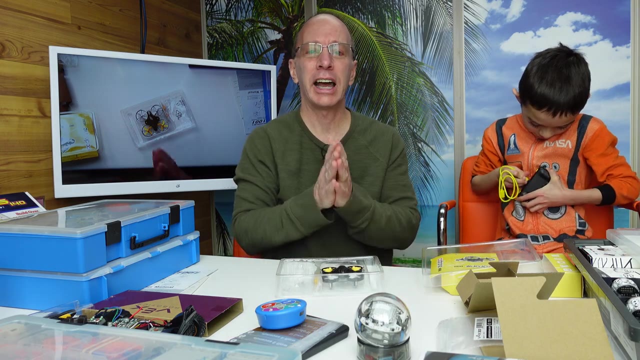 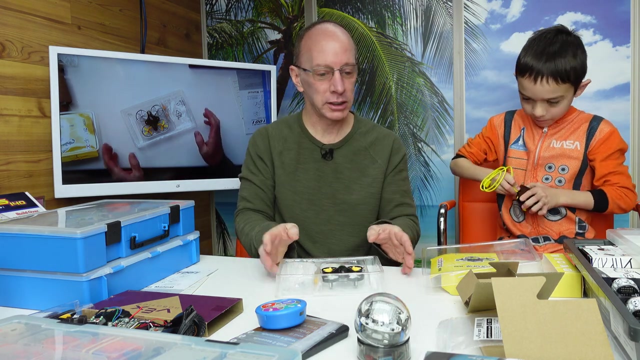 um, you hook it up through this control. uh, you can use this controller if you want to. um, but the students are going to have an awesome time programming this uh little drone. now this company is called robolink. check it out. they have bigger drones and more advanced um and for uh coding and programming. so all right, Lucas, I'm going to move on a little. 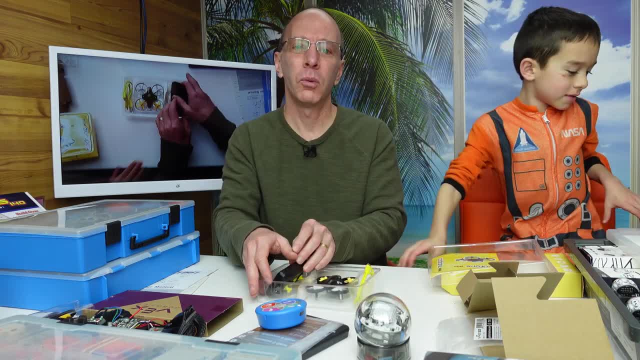 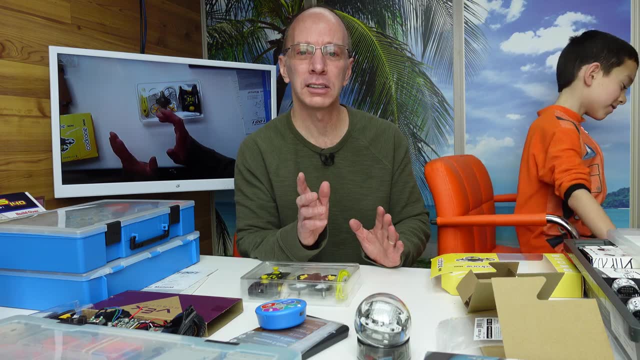 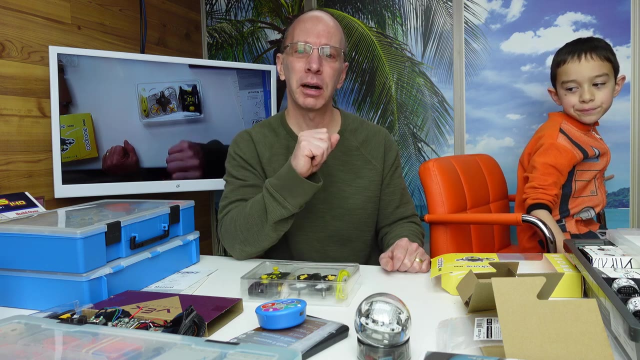 bit um with robotics, with programming. um, you got to make your own robot. yes, you want to start to make your own robots. um, there's also a website. it's, I think it's called, hour of code, I think it's called. I'd recommend that because it really gets the kids excited and learning about coding. they have some. 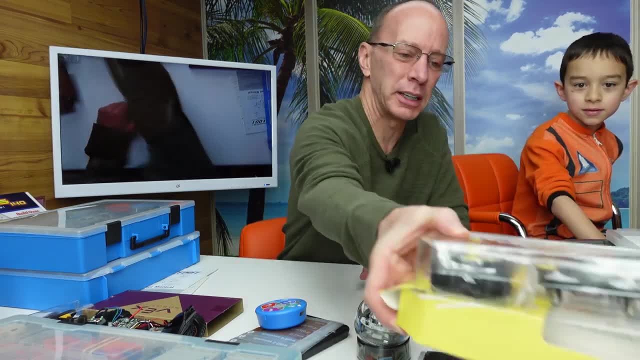 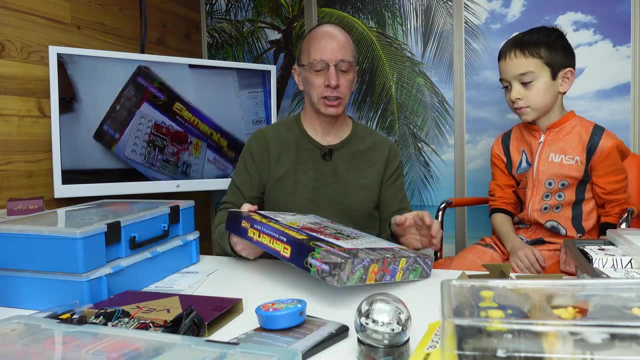 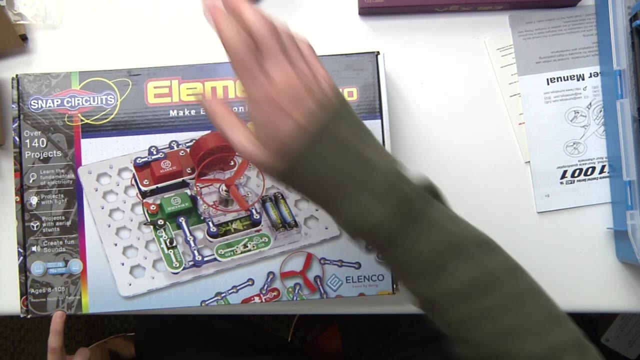 awesome tutorials on there and running out of table space right here and you want to start getting more into electronics, um wiring, um circuitry, um kind of pushing your class toward that again. working with vex, working with ozobots, you're, you're adding that that next level of 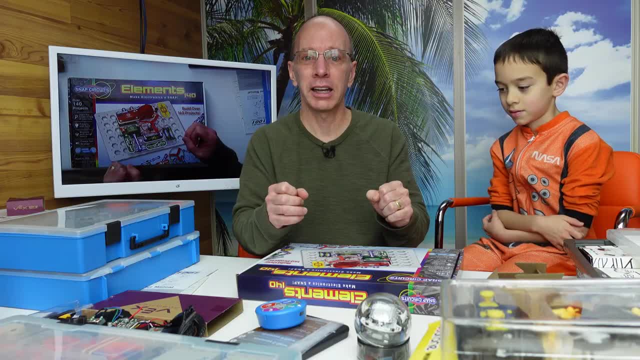 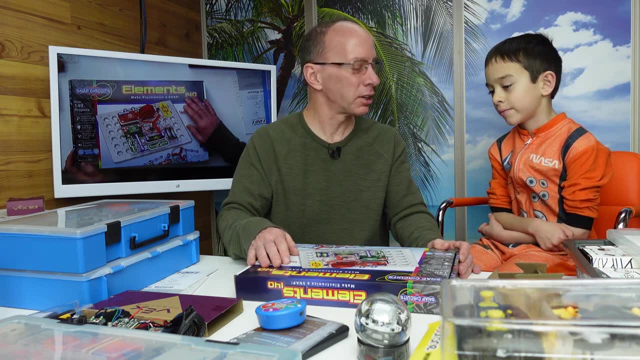 excitement and you can start to have the kids. you know the kids might like: hey, I want to start building my own robot. well then, let's start. you know work as a robotics teacher. let's start understanding some circuitry. so this is one. I did not have a chance to review this, or 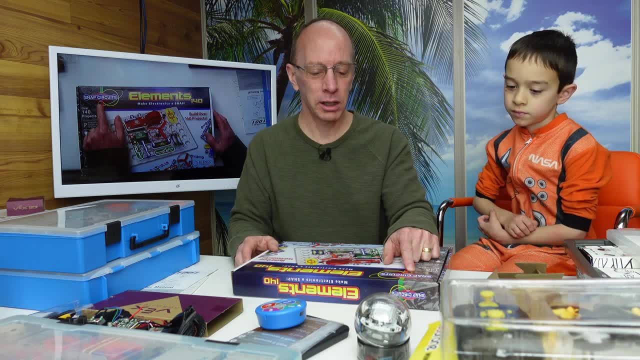 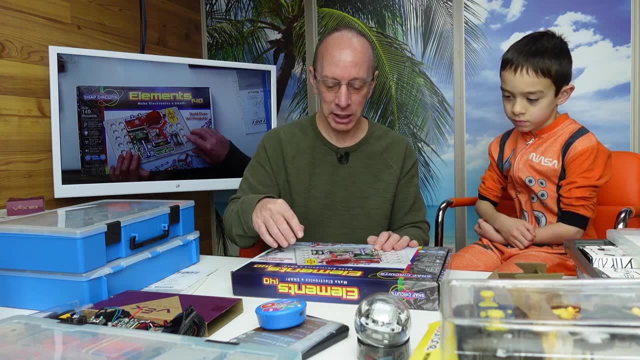 even take a look at it. the company I know is starting to work on a curriculum for teachers. I don't think they have it set up yet, but this is um one of my students. actually, her name is Lucy. she sent me um a video and she was working with. this is like hey, this is awesome. and she started 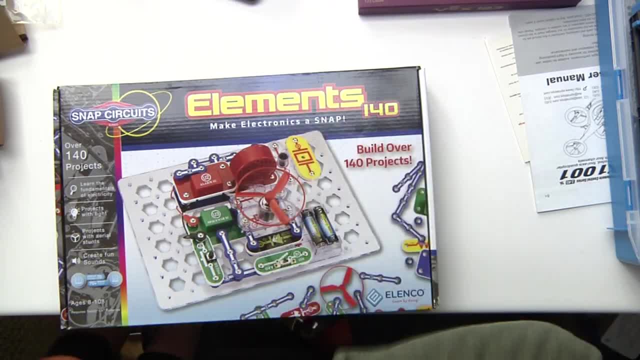 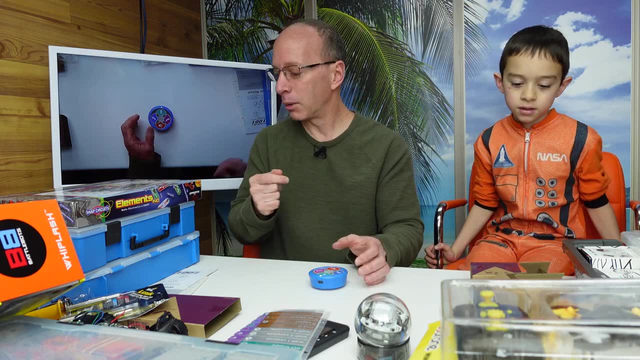 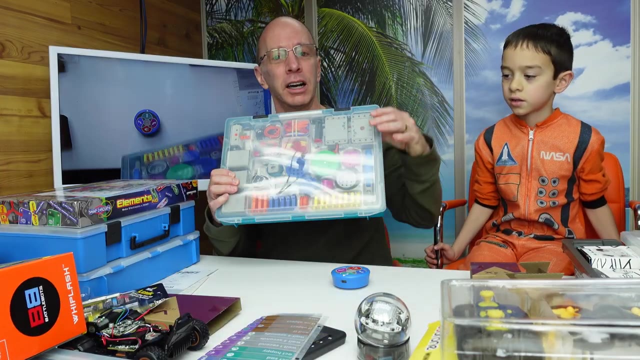 to understand circuitry that you have to have a closed circuit and creative and positive- so awesome. I'm starting to run out of uh battery time so I gotta really hurry up, so let's- um, okay, about 120 dollars. vex go right here. I'm teaching it in third grade. they love it.